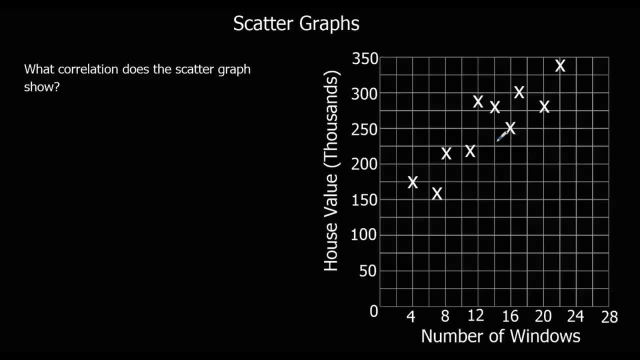 here we're looking at a relationship between the number of windows and the value of a house And the question says: what correlation does the scatter graph show? So what's the relationship here? So we can see there's a kind of an upwards trend. So we've got the points following. 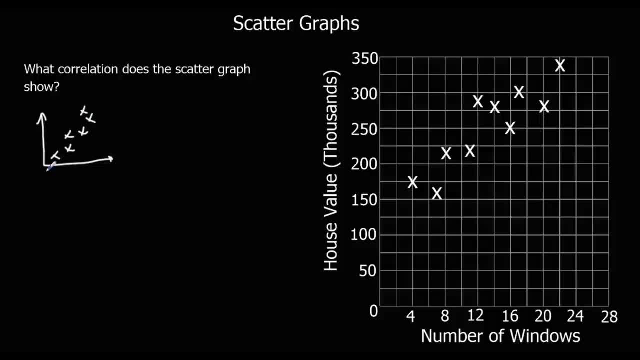 this kind of direction. That means as the number of windows goes up, the value of the house goes up, And that's called a positive Positive correlation. Positive correlation If it was going down. so if, as the number of windows increased, the house value decreased and it followed like a downwards line, that 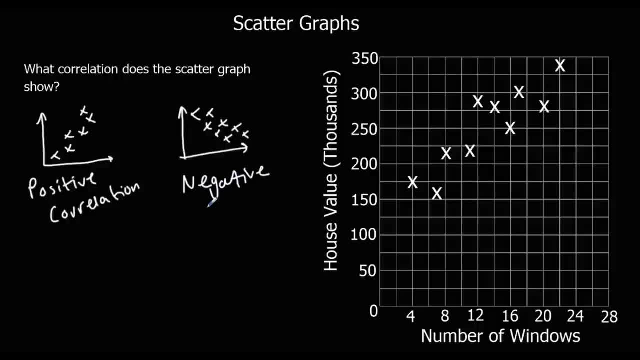 would be called a negative correlation. Negative correlation. And if the points were all over the place and there wasn't a real pattern, so like that, that would be no correlation, No correlation. So we need to be able to look at scatter graphs and look at the relationship. 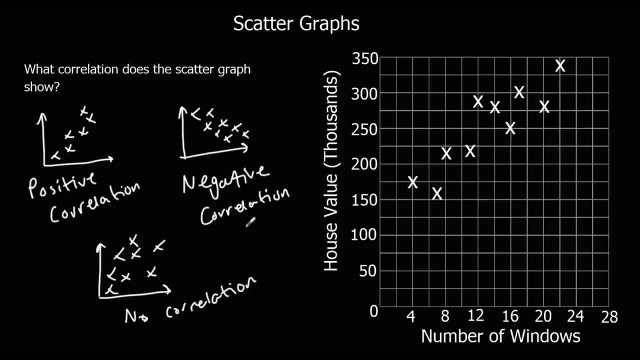 between them. So we can say, as the number of windows increases here, the house value also increases. It's important to note, though, that just because it's a correlation, it doesn't mean that there's causation. So it doesn't mean so correlation, correlation does not. 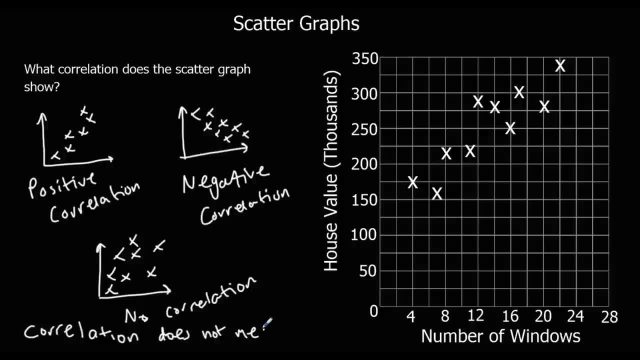 mean Causation, Causation. So just because as the number of windows goes up as a pattern, the house value goes up, it doesn't mean the number of windows causes the house value to go up. So if I decided to put 10 new windows in the same house, thinking that'll increase, 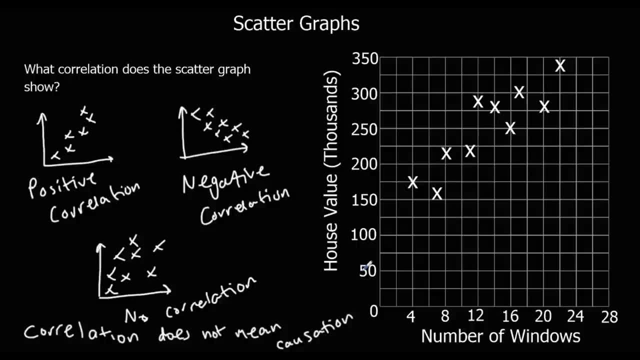 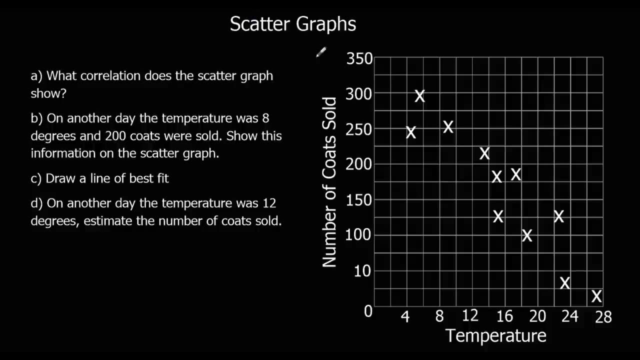 the house value. it'll probably look silly, and it probably won't. So correlation does not mean causation, It just means that there's a relationship there. So here's a question. So what type of correlation does the scatter graph show? firstly, Well, 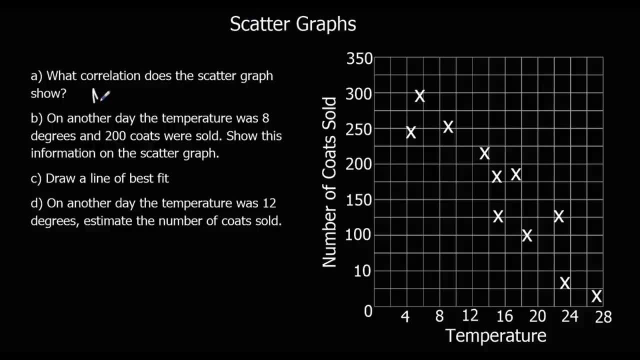 it's going down. It's a negative correlation. It's going down, So negative correlation. And if I wanted to describe the relationship, as the temperature increases, the number of coats sold decreases. So on another day the temperature was 8 degrees and 200 coats were. 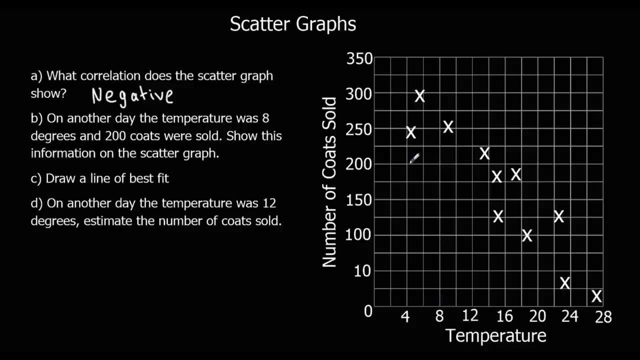 sold. So 8 degrees, 200 coats. We're going to show this information and that's just going to be an X, 8, 200.. Draw a line of best fit. So what we need to do is we need to draw a line roughly going through. 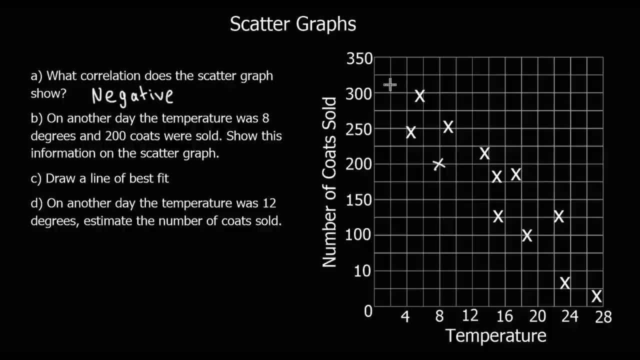 the middle of the points. So here I can get six points on both sides If I do a line down there, maybe angled a little bit, Yes, So what we're trying to do is get the least distance from the Xs through the lines. So 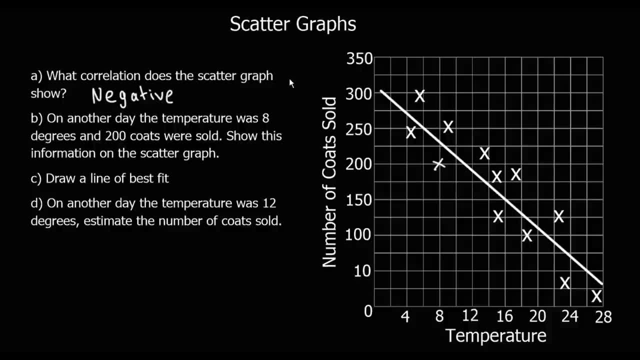 the line that best fits these points. So if we've got 6 on both sides, it goes roughly through the middle in the same direction. That's a good line of best fit, So we've done that. On another day the temperature was 12 degrees. Estimate the number of coats sold. 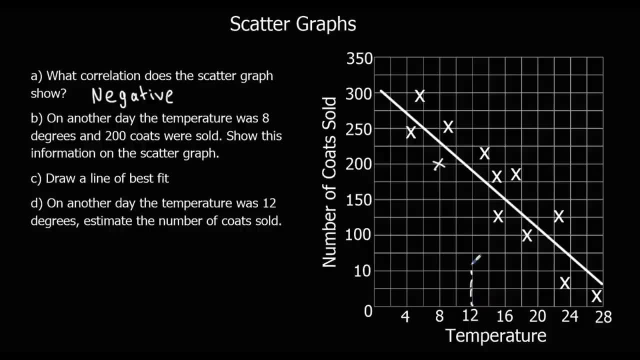 So 12 degrees is here. We go up to that line and then across. Across from our line. It's going down and then across. It's going down, Then across from the line And then across line. now we should use a ruler here and I can't do that, so I'm just gonna do the 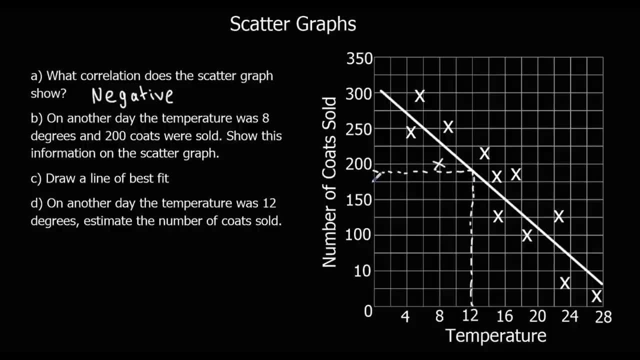 best thing I can with my eye. and and that's 175 there, so that's 175. let's say it's a roughly 190, roughly 190 coats. there'll be a margin of error in an exam that you're allowed to have an answer between something and something, and so 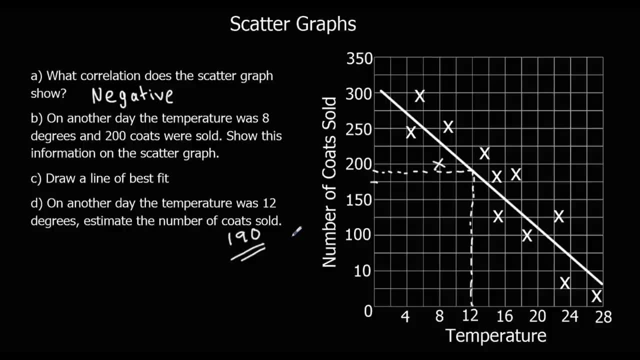 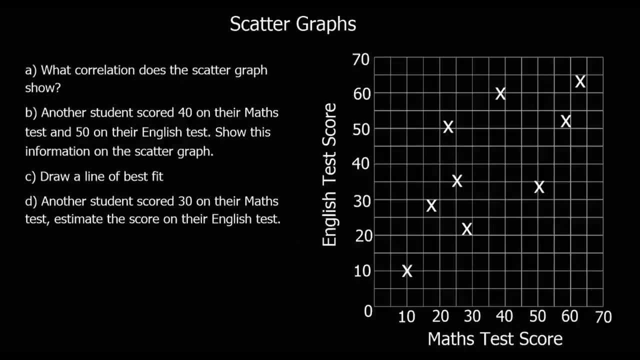 as long as you draw a good line of best fit. it goes through the middle of the points and your answer should be within them, within the range. okay, here's another question and pause the video and see if you can give it a go. okay, so the correlation here? the correlation here is positive as the math.